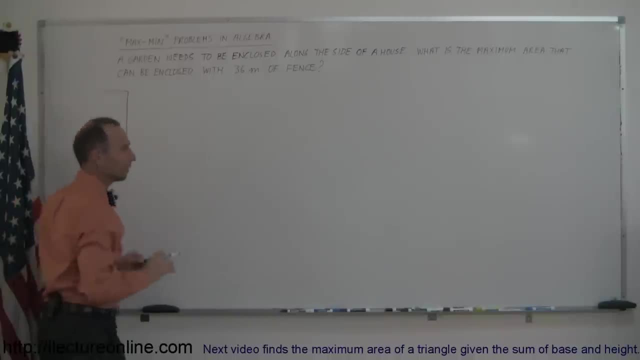 here's the house, and this is kind of like a bird's eye view picture- and then we're going to draw a little drawing here, and then we're going to draw a little drawing here, and then we're going enclose a garden with a fence like this. 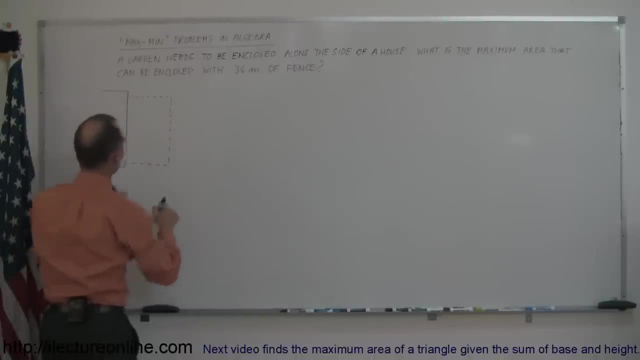 and, of course, we don't need to use a fence. on this side we already have a house. so for three sides of the area that we're going to enclose, we need to use the fence, and we only have 36 meters of it. So let's say that this side over here, this is X. 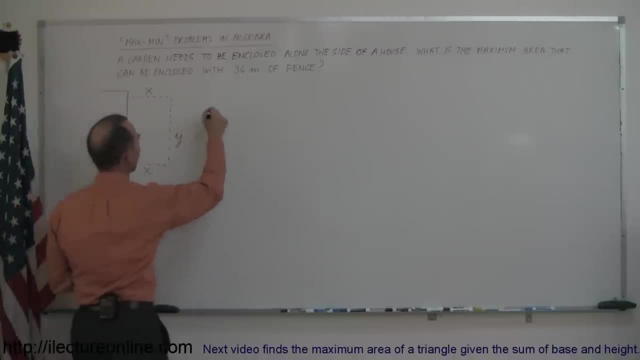 and this is X and this is Y. we can then say that the area area is equal to X times Y- length times the width, and we want to maximize the area. so we need to come up with an equation that allows us to find the the area, and it needs to be a quadratic equation, of course. you can only have one. 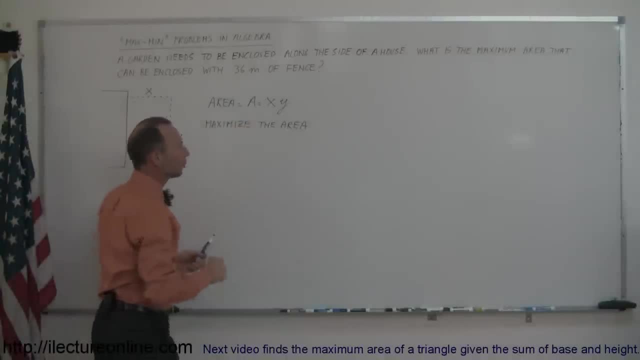 variable. here, A, can only be dependent on either X or Y, so we need to find some constraint. so the first thing we do is find an equation. the second we do is realize what we're going to maximize, and then the third thing we need to do is we need to express the equation in terms of only one variable, in this case, 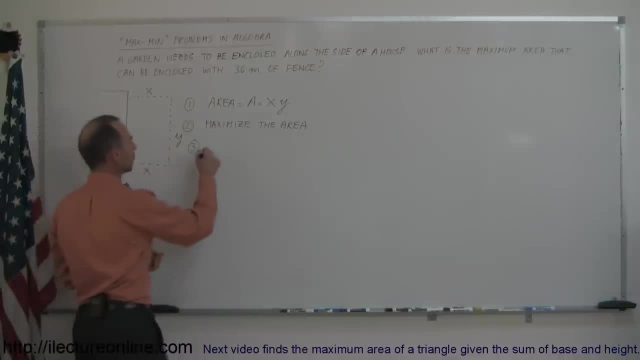 we have two variables, X and Y. so we're looking for a constraint, so we're going to use a constraint. in this case, the constraint is that we only have 36 meters of fence. 36 meters of fence, that's the constraint to eliminate one of those two variables. 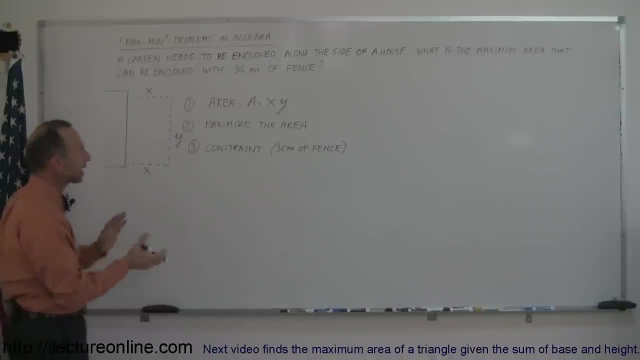 so we need to be able to use this information to express X in terms of Y or Y in terms of X. so here you can see that if we add X plus Y plus X, that should add up to 36, so we can say that 2x. 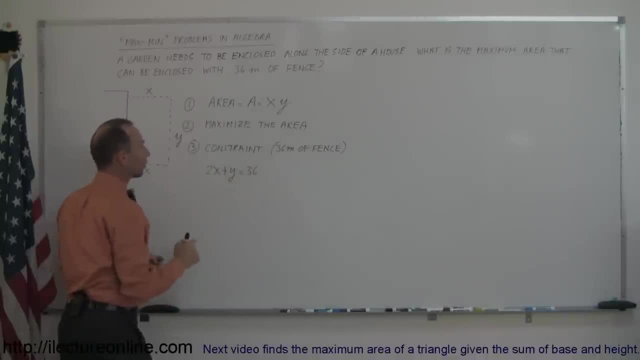 plus Y equals 36, which means I can replace the value for Y by 36 minus 2x by bringing the 2x over to the other side and substitute that into my original equation. we now developed the equation with only one of the two variables, so now we can. 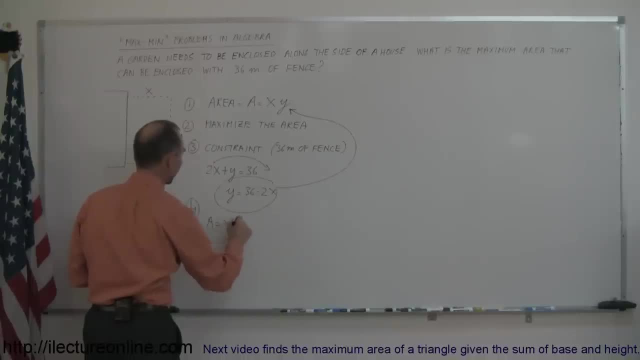 say that the area is equal to X times Y, but instead of Y we're going to write what Y is equal to, which is 36 minus 2x, and if you multiply this out we get: area is equal to 36x minus 2x squared. 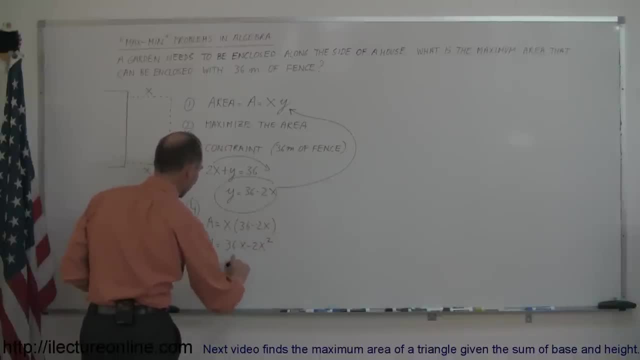 or, if I rearrange it, I can say: A is equal to minus 2x squared, plus 36x minus 2x squared. all right now, since this is a negative x squared, or, in this case, negative 2x squared, we can imagine. that's a parabola which is: 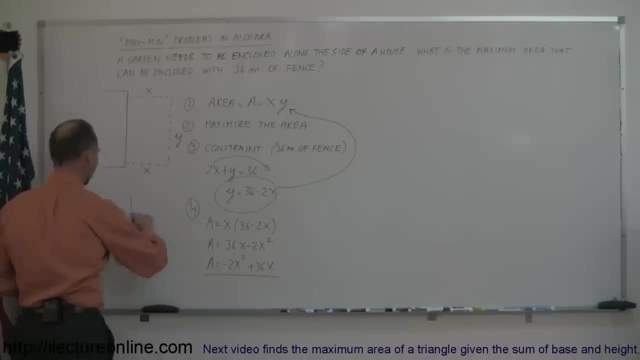 if we were to graph that, or at least sketch it, that it looks something like this: so the parabola will open downward and that means that we have a maximum value on this parabola. so we want to find the highest value in the parabola, which means we want to find the 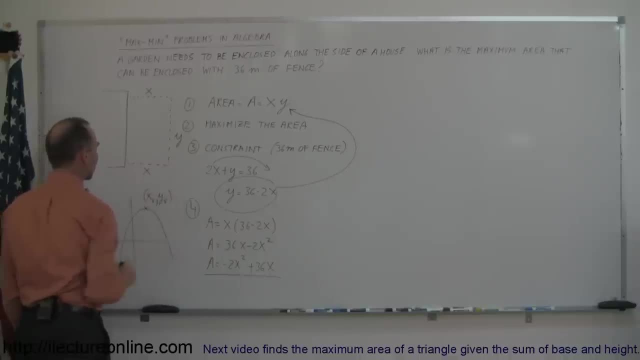 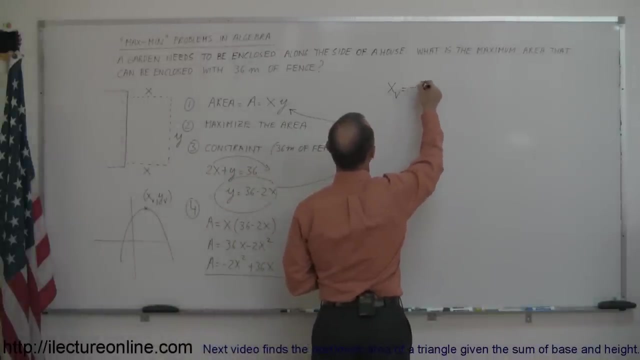 vertex X sub V, Y sub V on that parabola. so at what point do we have the highest point on a parabola, the vertex, and from remember right from elsewhere, we can say that the X sub V is equal to minus B over 2A. 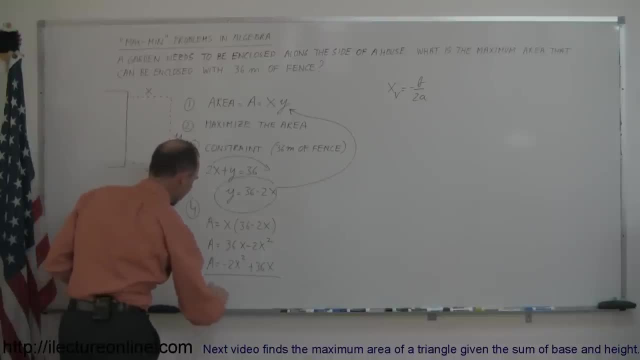 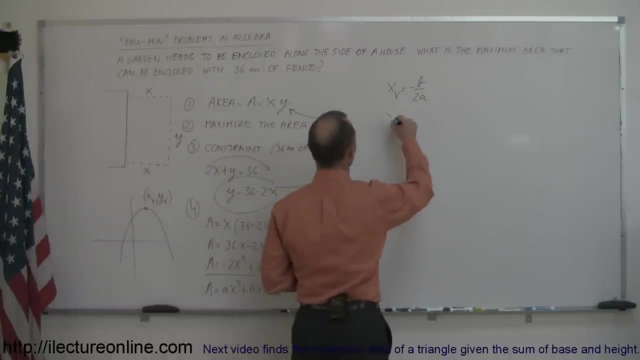 so remember that general quadratic equation we have: Y equals AX squared plus BX plus C. so minus 2 would be A, 36 in this case would be B, and if we plug A and B in that equation we find the X value of the vertex. we can say that X sub V is equal to minus B and 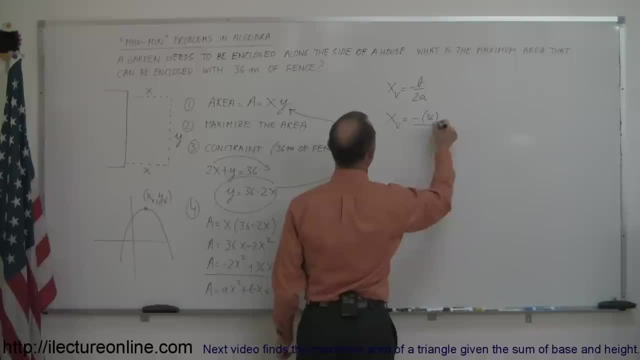 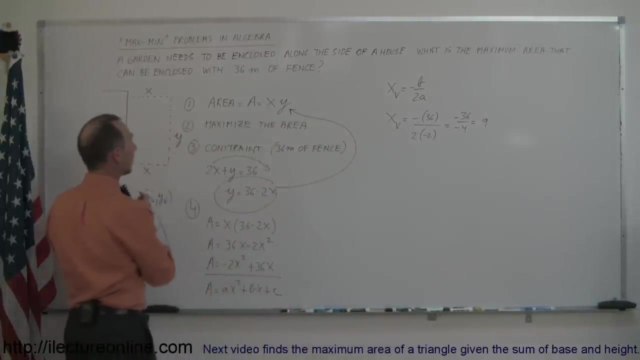 B is 36, that's minus 36. divided by 2 times A, which is minus 2, that gives us minus 36 divided by negative 4, which is a positive 9, which means that for us to find the largest area, X has to be 9. 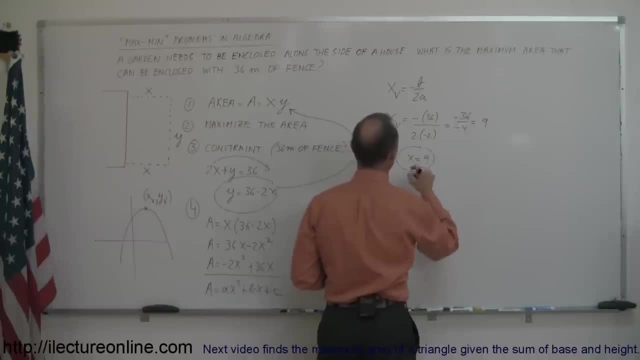 So therefore we conclude, x must equal 9.. And so once we know what x is equal to, we can plug that into our constraint right here to find the other variable. So come back over here. We'll say: y is equal to 36 minus 2 times x and x is equal to 9.. 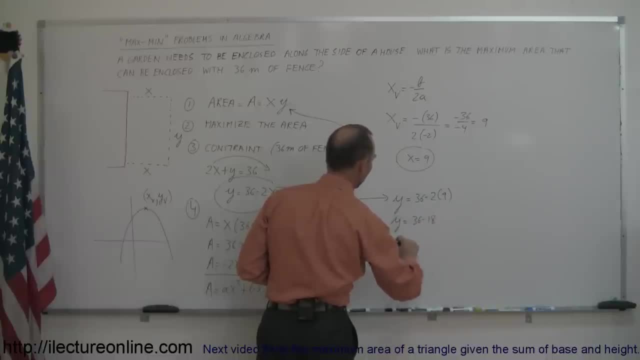 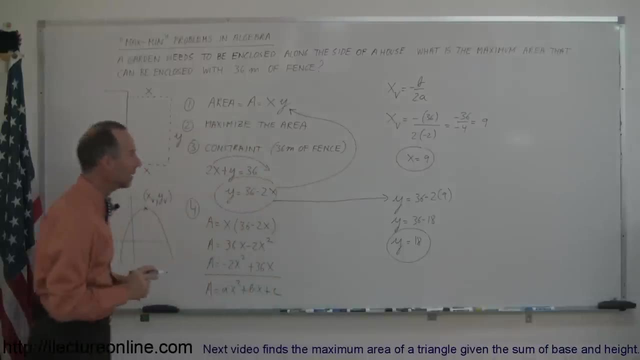 So y is equal to 36 minus 18, and y is equal to 36 minus 18.. That would be 18.. So the maximum area can be made when we let the width equal to 9 and y equal 18.. Okay, now what's the area then? 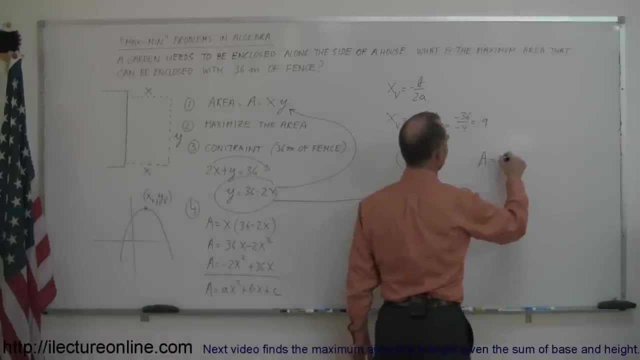 Well, we have the equation: area is equal to x times y, So area is equal to 9 times y, which would be 18.. And so a is equal to 90 plus 72, which is 162.. And of course, the units would be square meters. 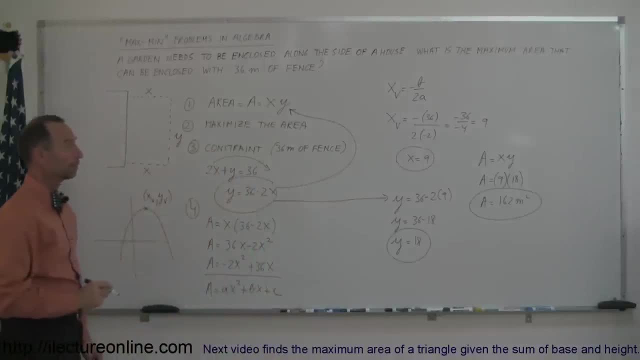 So that's how you find the maximum value using algebra. Let's do a quick review of that. So you were given a problem where you had to make an enclosed area using 36 meters of fence, using the wall of a house as one of the sides. 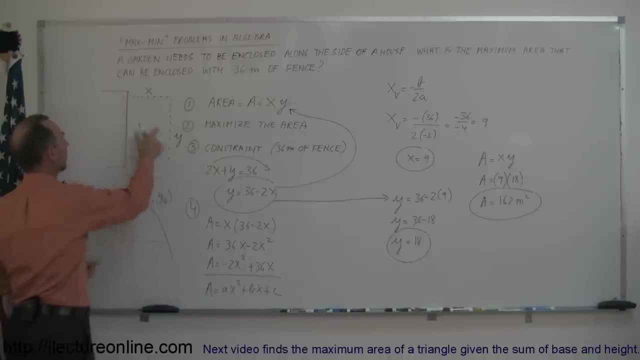 which means you'll have a width and a length of that area, And the width can be set equal to x, The length can be set equal to y And then the area simply would be x times y, which is your equation That gives you the area. 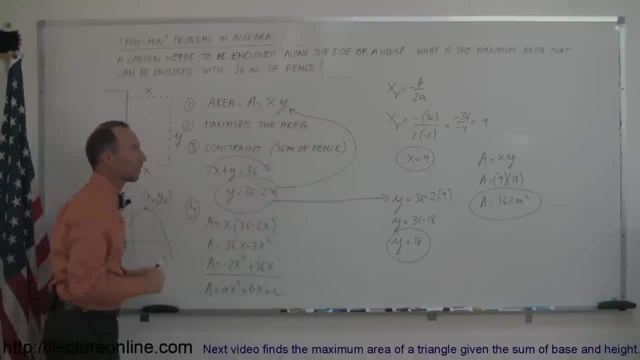 But as you can see that the area was given in terms of two variables, You need to realize, then, what you're trying to maximize, And this is the area. In this case, you're trying to maximize the area, And then you need to come up with a constraint. 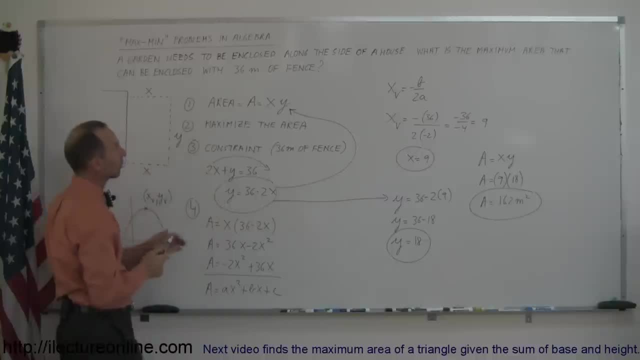 some sort of relationship between the two variables so you can eliminate one of the variables. The constraint here was that you only had 36 meters of fence. Looking at the drawing, that meant that x plus y plus x cannot be any bigger than 36.. 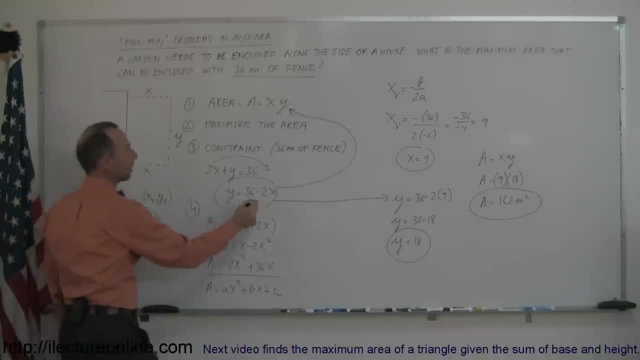 So 2x plus y is your constraint. You solve that for y, Plug that back into your original equation for the area. So then you end up with just an equation. Where am I here? Oh, there we go. y is equal to this. 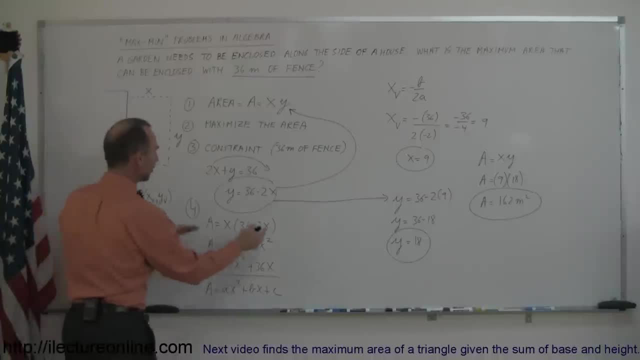 There we go, 4.. I kind of lost myself here for a moment. So then I end up with the same equation, but instead of writing y, we write what y is equal to in terms of x, And now you can see that you have a quadratic equation. 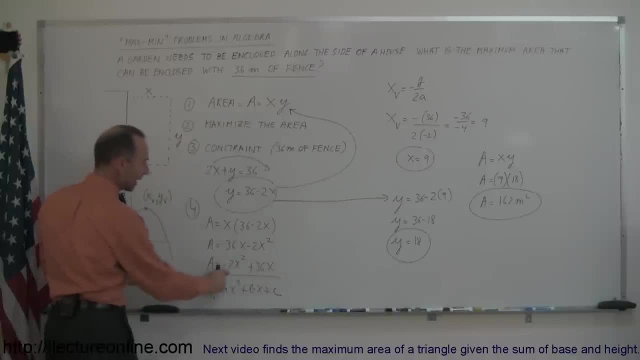 Realizing that the first term, the x squared term, is a negative. we know, then, that we have a parabola that opens downward, which means we have a maximum value on our parabola here at the vertex. We realize that. 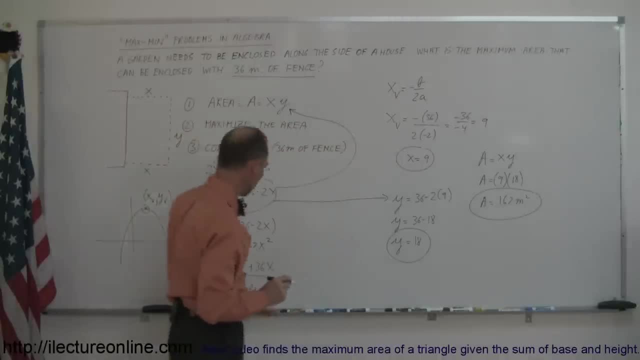 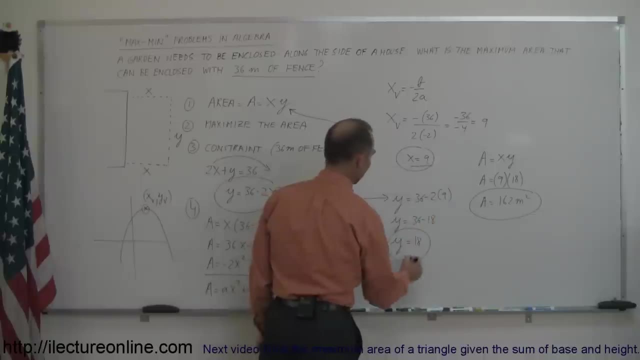 To find the vertex of a parabola that's equal to minus b over 2a, based upon what our general equation is of a parabola. And then, when we plug in the numbers, we get a value for x, we get a value for y and we can calculate the area. 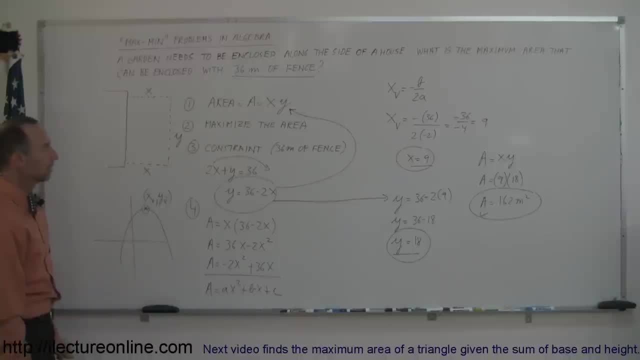 And that's how you solve a problem like that. All right, Hope that helps. I'll do a few more examples of this.